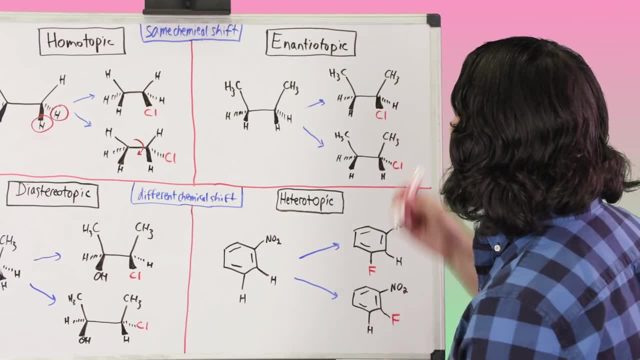 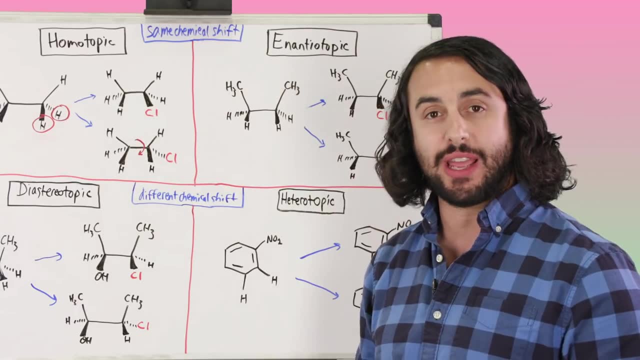 So what does enantiotopic mean? And so let's perform the exact same thing. Let's notice here that instead of ethane, we're actually looking at butane, So we have these two methyl groups there instead of hydrogen, And we'll do the exact same thing. 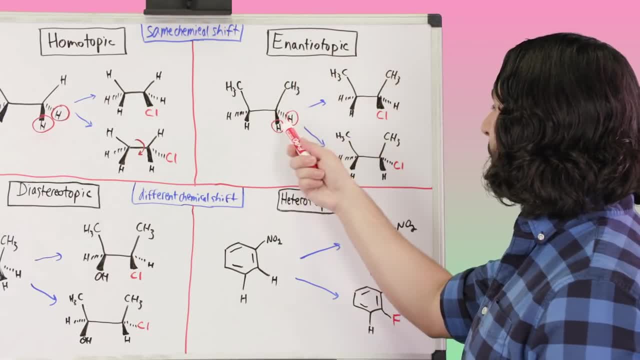 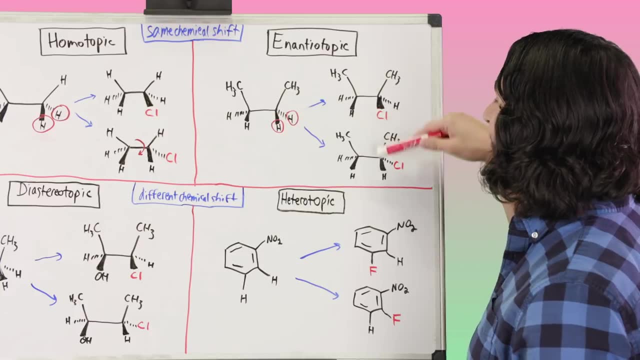 We will compare these two hydrogens and on the top one we'll turn the one on the wedge into chlorine. on the bottom, we'll turn the one on the dash into chlorine. Now let's compare the relationship between these two molecules And actually in this case we are generating a chiral center. 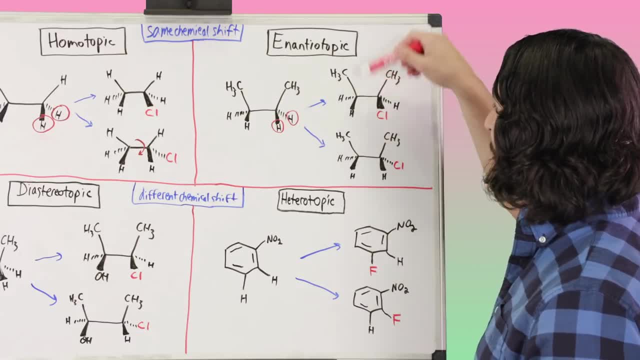 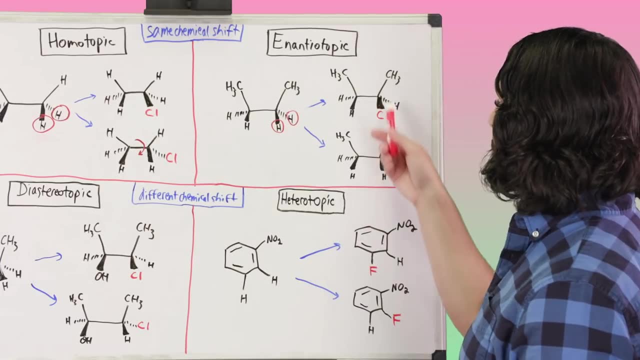 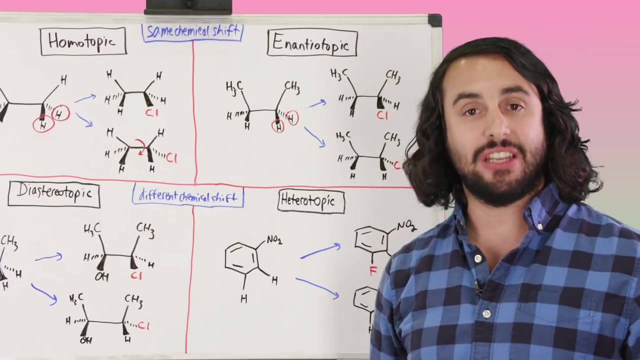 Because there are four different groups. We've got methyl hydrogen, chlorine and the rest of the molecule and in fact we are generating the opposite stereochemistry at this center, depending on which hydrogen we turn into chlorine. And so, because these two molecules are enantiomers of one another, the relationship between these 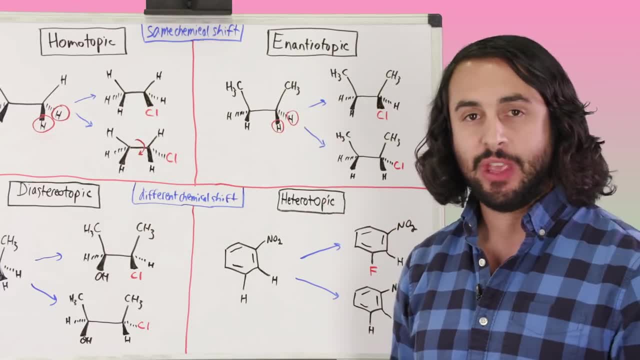 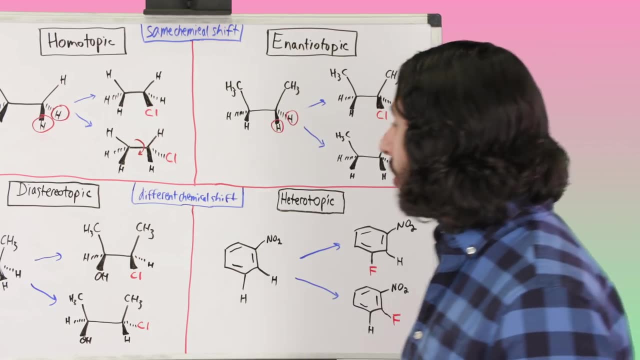 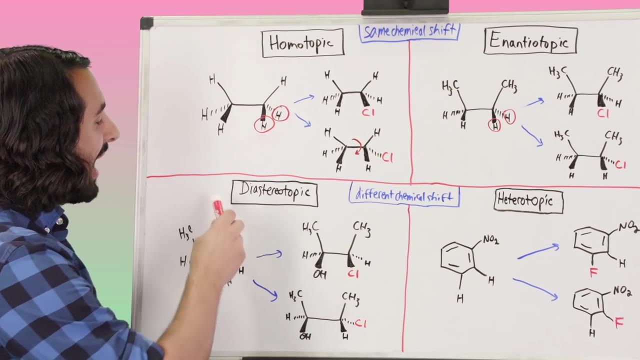 two protons is an enantiotopic relationship, So these are enantiomers. therefore these protons are enantiotopic. As you can guess from the pattern here, probably we're getting to diastereotopic. And so now, with diastereotopic, let's notice the key difference. here we've actually 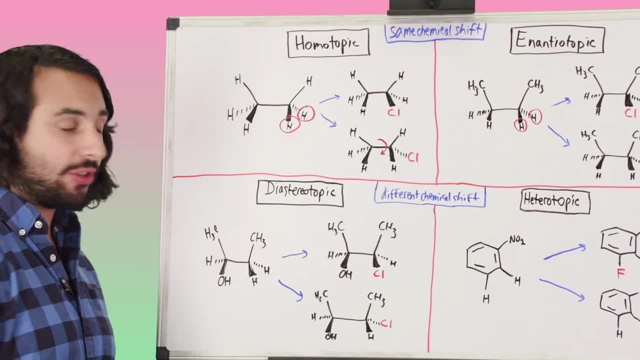 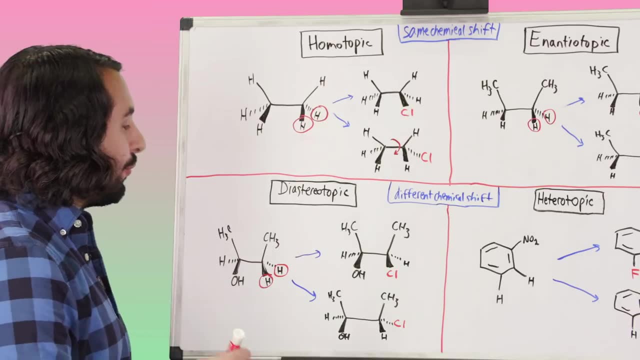 added a hydroxyl group right there on the wedge of this carbon, right here, and we're gonna do yet again the exact same thing. we're gonna take these two hydrogens and for one molecule we'll turn the one on the wedge into chlorine, and for the other one we'll 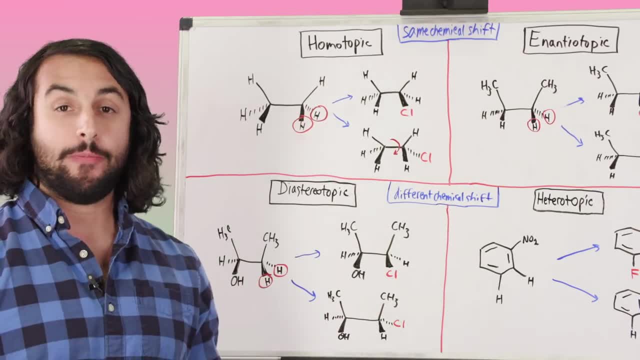 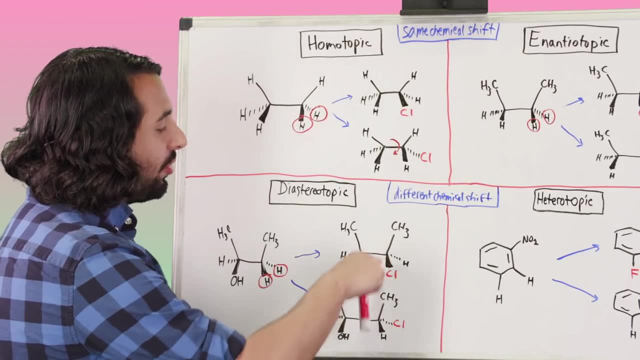 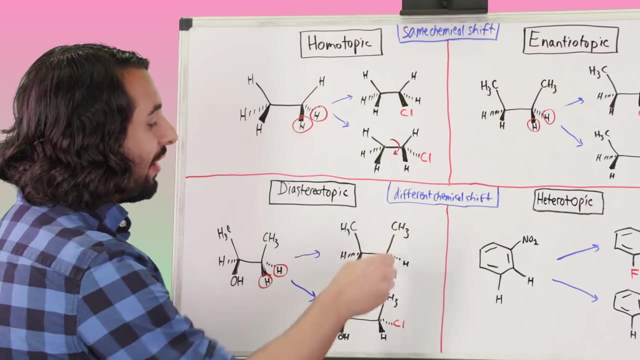 take the one on the dash and turn that into chlorine. This is a different situation than for enantiotopic, because it is true that we are generating a new chiral center and it is true that we are generating the opposite stereochemistry at that new stereocenter, depending on which one we turn into chlorine. 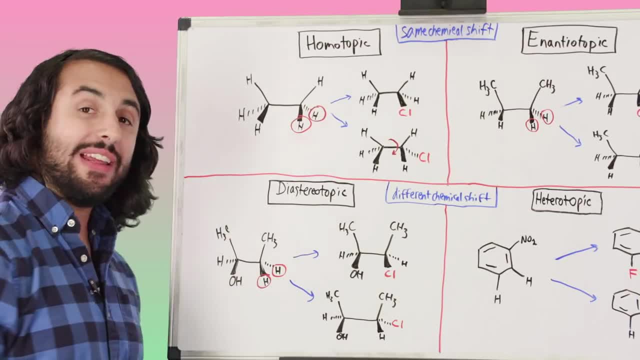 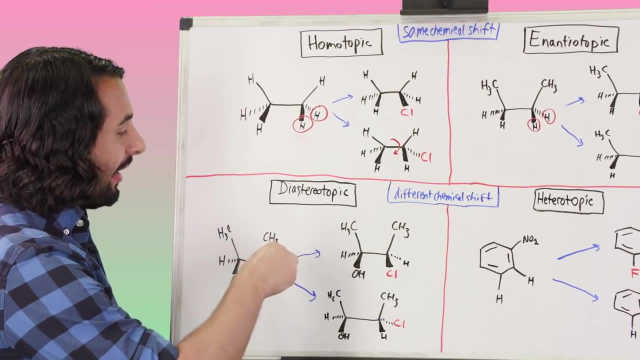 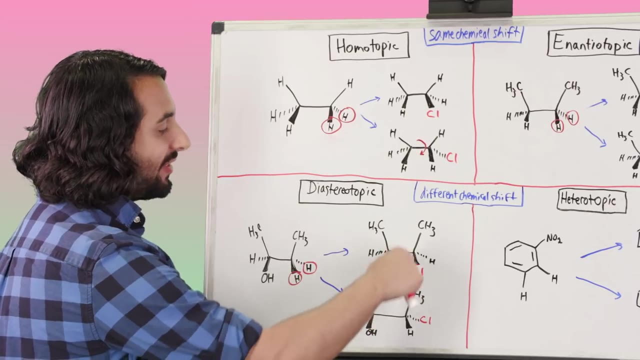 But there is a pre-existing stereocenter. This carbon right here is also a stereocenter and that stereochemistry is not affected. it is not altered by this activity. right here This stereocenter stays the same, but we have a new stereocenter that is opposite, depending. 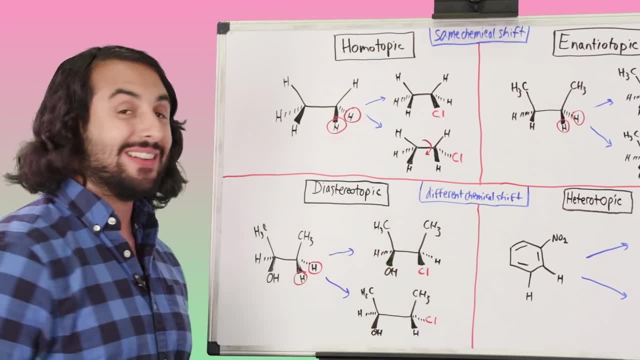 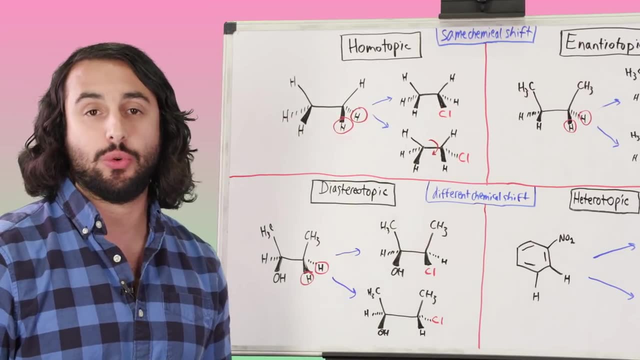 on which one we're looking at. We are actually generating two different diastereomers. right, These are not enantiomers of one another, because recall that diastereomers are molecules where one, at least one, but not all- of the stereocenters are inverted. 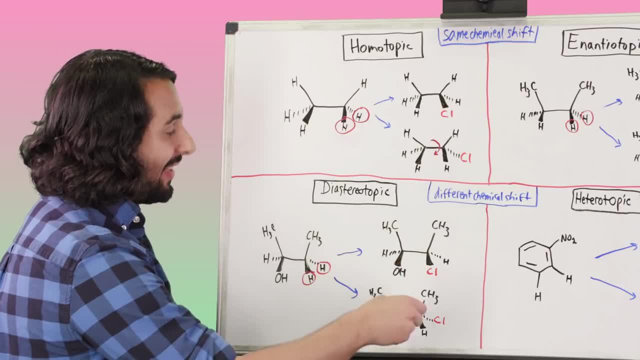 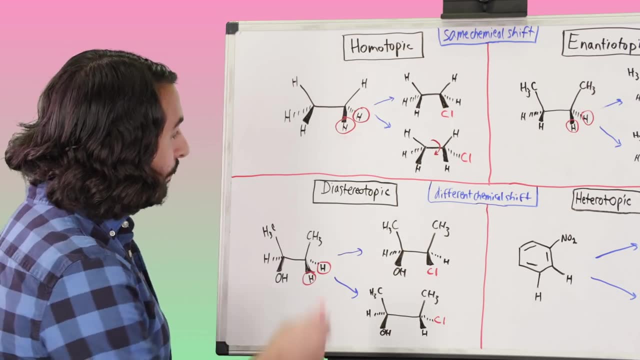 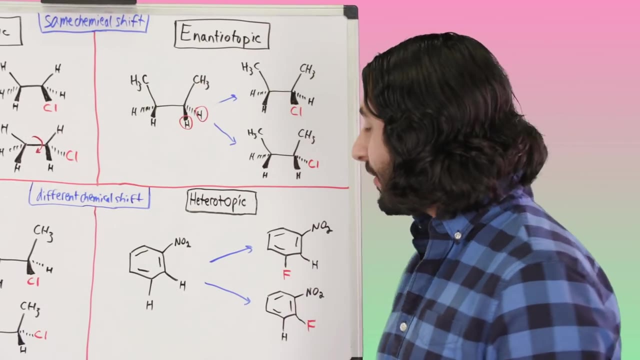 So this stereocenter is inverted, but not this one. so these are diastereomers of one another, and therefore these hydrogens have a diastereomers. And so that's these three, let's round it off here. And the last one is heterotopic, and so heterotopic is a little bit different, and so let's say: 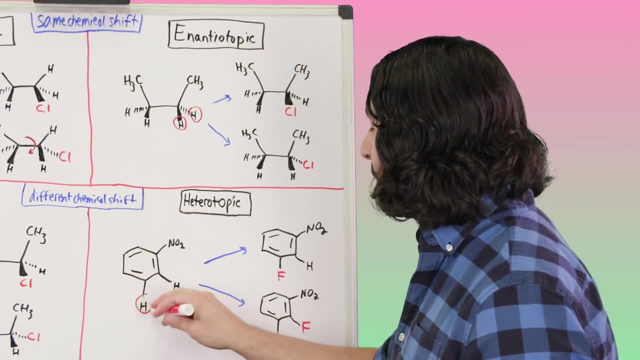 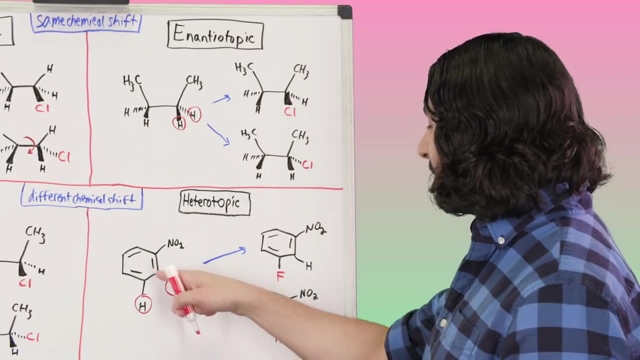 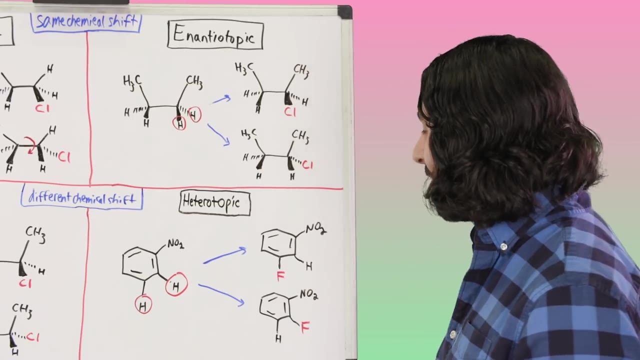 we've got this nitrobenzene and we'll arbitrarily look at these hydrogens. we could be looking at any of them, but we'll take a look at these two and on this one, let's take the bottom hydrogen right here and turn that into fluorine- again arbitrarily. could be any other element. 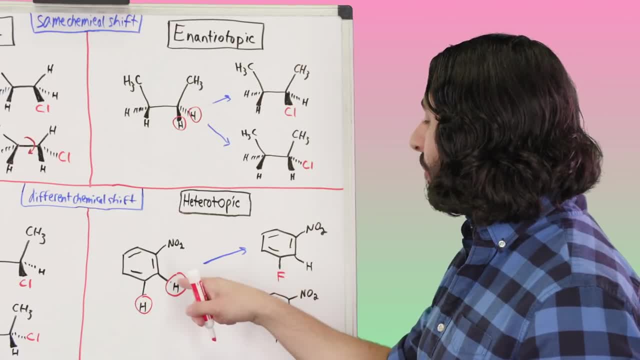 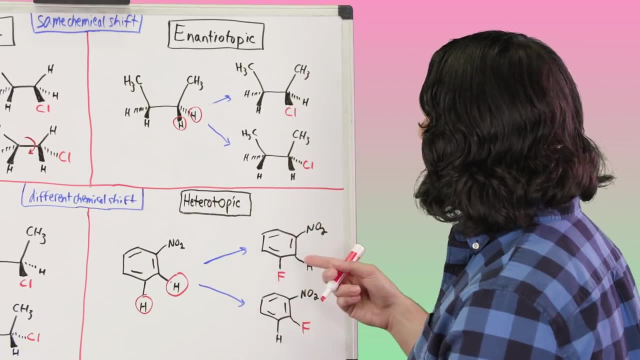 but we're just saying we're going to change this one into fluorine over here, and then we're going to change this one into fluorine over here, And now we're going to compare these two molecules And what we see is that these are no longer mere stereoisomers of each other. these are 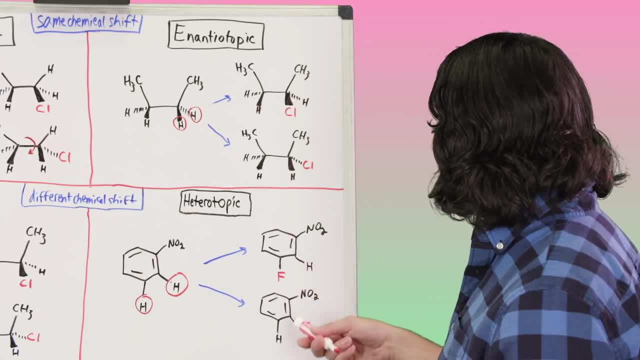 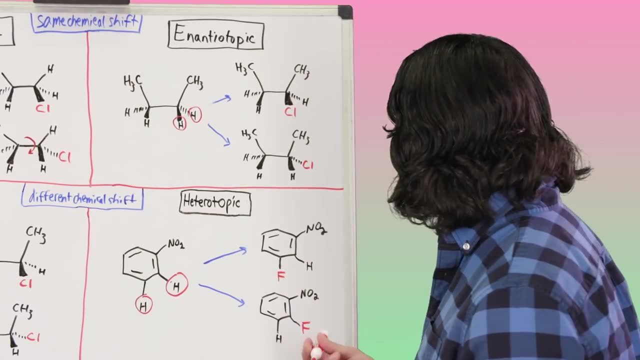 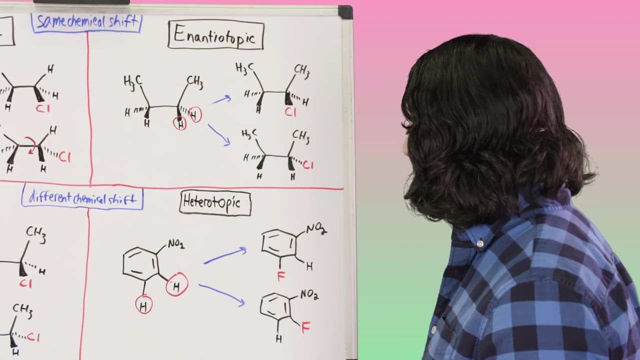 actually structural isomers of each other. These are completely different molecules because the position of the fluorine is in a different location and so this is actually going to make these protons. that means these protons have a heterotopic relationship And so we've got these molecules are the same homotopic. these molecules are enantiomers. 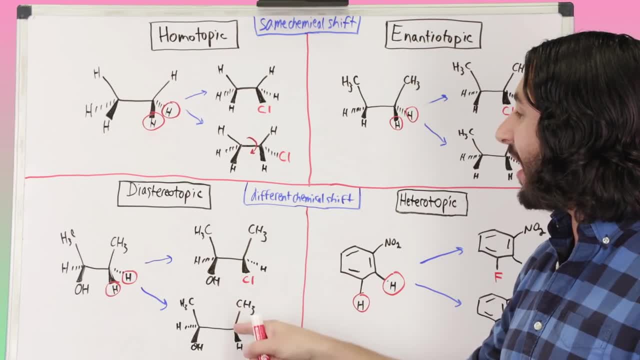 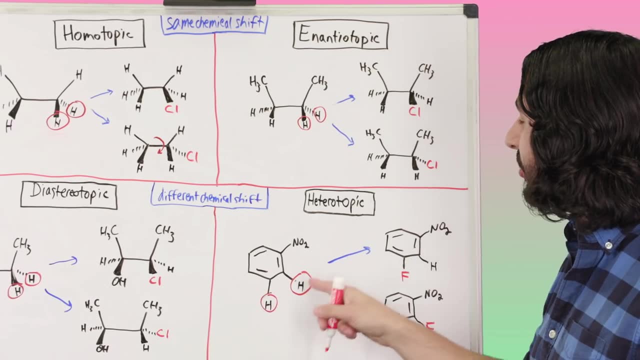 so these were enantiotopic. these molecules are diastereomers, so these were diastereotopic. and these are structural isomers of one another, so these hydrogens are heterotopic. So hopefully that makes the definitions of these words pretty clear. 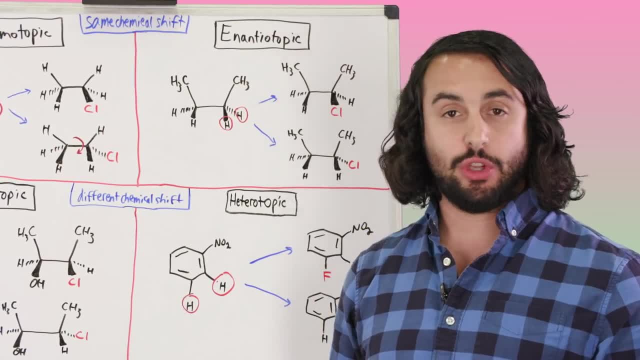 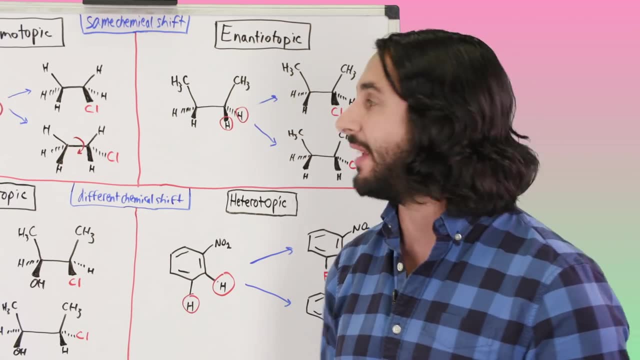 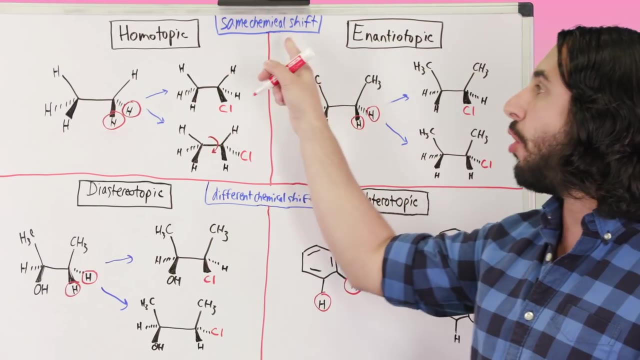 Before we move on, let's just point out one other thing, Because this is used often in the context of NMR spectroscopy. one thing that we want to understand about the chemical shifts of these kinds of protons is that anytime you have homotopic or enantiotopic protons, these will all have, they will all show the same. 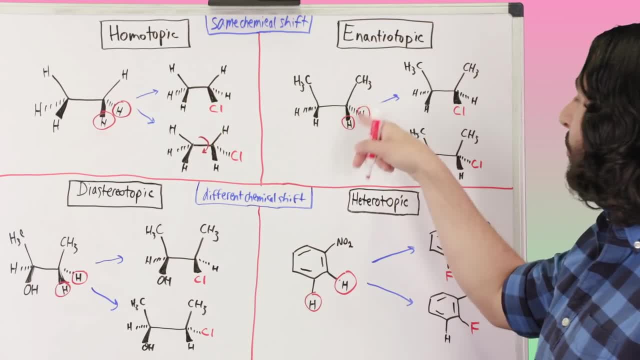 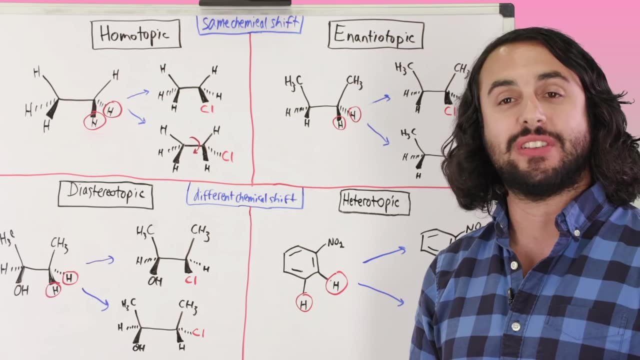 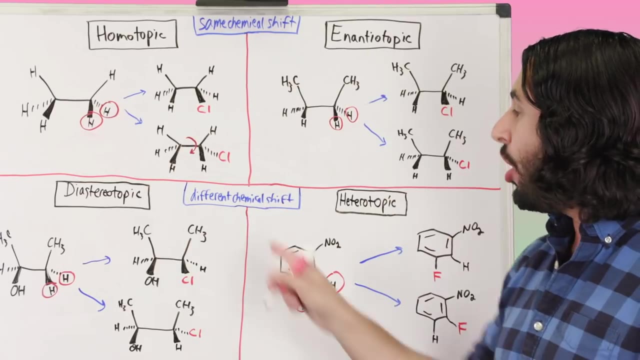 chemical shift. So these protons and these protons will all show up on an NMR spectrum with exactly the same chemical shift because of the way that they're experiencing exactly the same chemical shift. On the other hand, diastereotopic and heterotopic protons will show up with a different chemical. 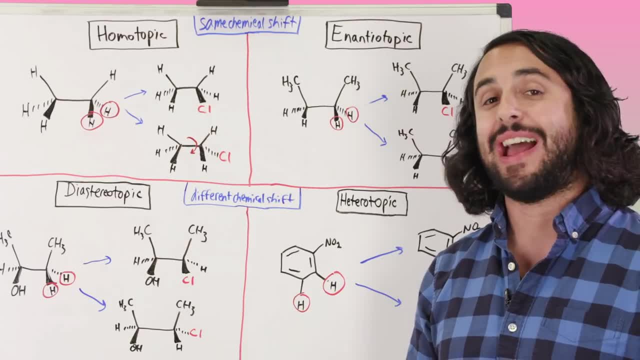 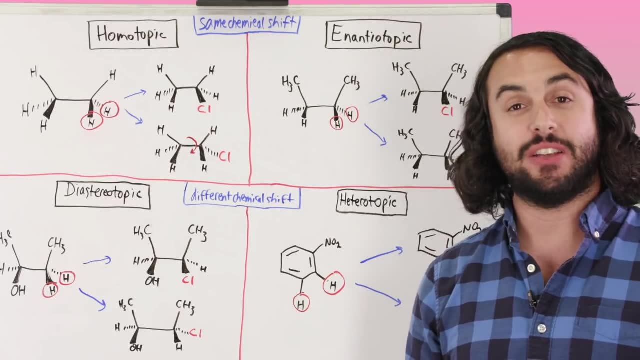 shift. so this is very important to understand because it's going to help us interpret NMR spectra. So this is not too difficult to see, because these hydrogens are actually occupying different positions on the benzene ring. so that seems relatively intuitive how these could show. 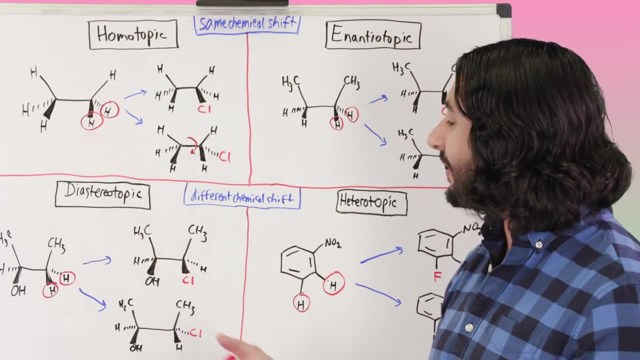 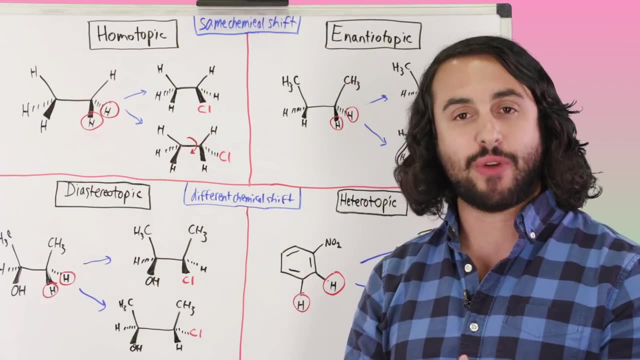 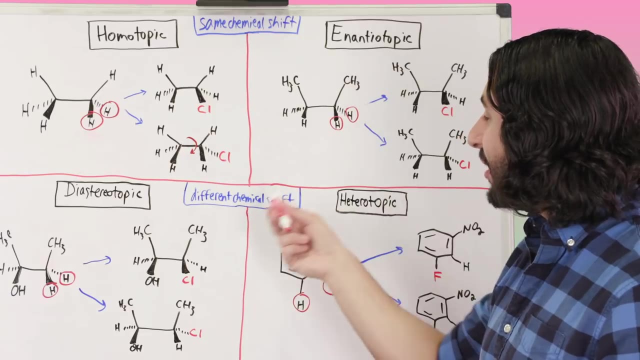 up with a slightly different chemical shift For diastereotopic. it's a little bit harder to see but just in terms of the spatial orientation of the groups they are experiencing a slightly different chemical environment at any given time. So same chemical shift when protons have this relationship and different chemical shift. 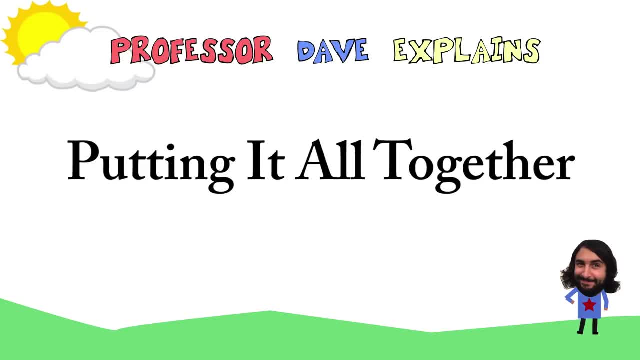 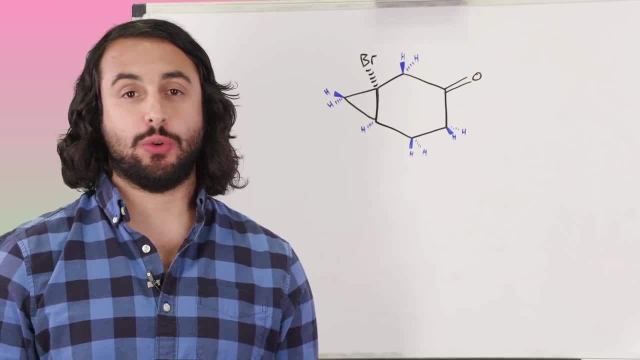 when they have one of these two relationships. So to put this into context, let's look at one example molecule and see what we can assess here. So let's say we have this interesting compound with a six-membered ring and then another. 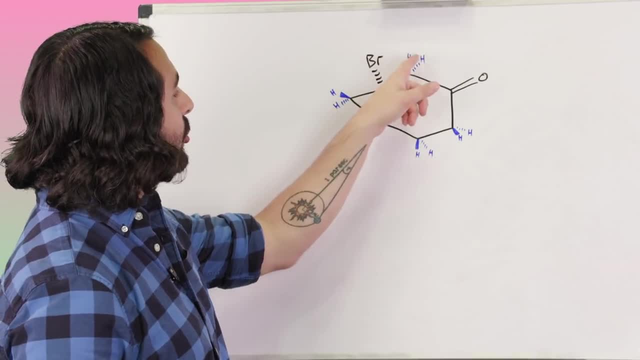 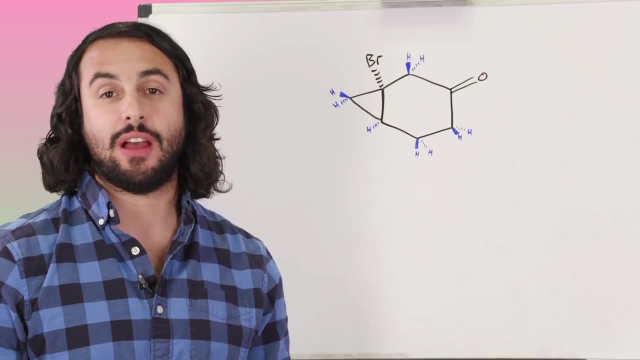 three-membered ring Right there, and so let's count up the hydrogens. we have two, four, six, eight, nine. we have nine protons here. what could we say about the relationships between any pair of these protons? and so, obviously, if we are examining protons a, 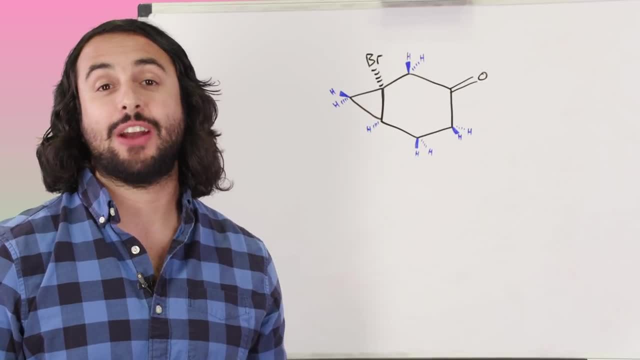 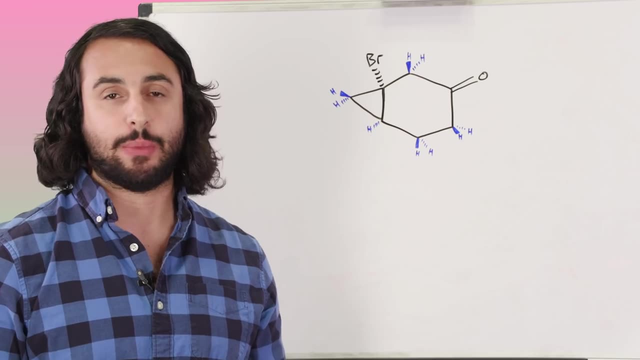 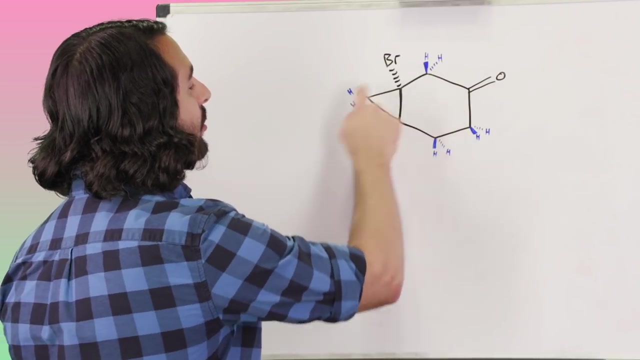 pair of protons on different carbons. those would all be heterotopic because in replacing those hydrogens by some other element we would definitely be creating different structural isomers. but for any of these carbons, for any of these pairs of protons, let's say we took these two or these two or these two. 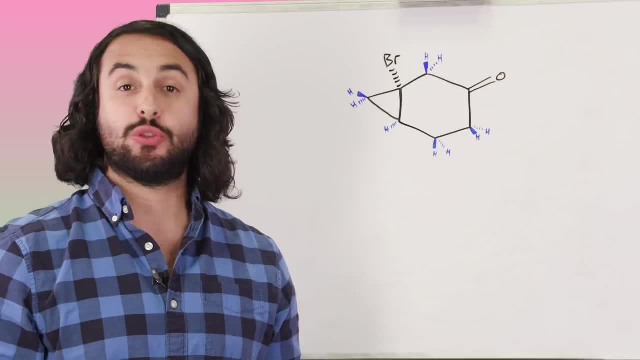 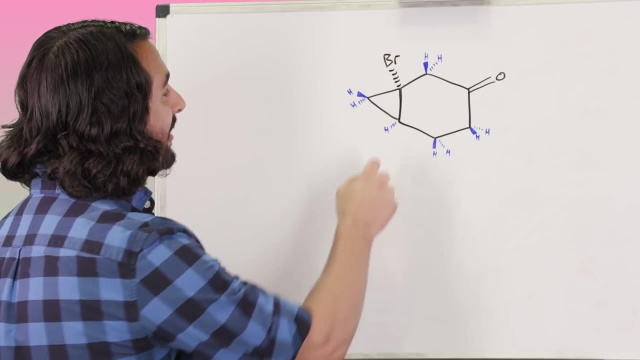 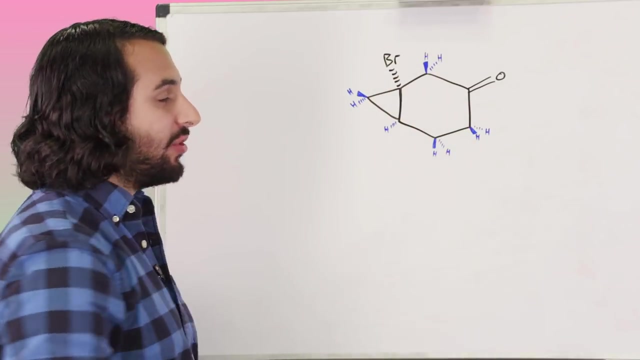 or these two. if we were to examine the relationship between those pairs, we would find that all of those pairs of protons are diastereotopic. so the reason is because of this existing chiral center right there, because we have a bromine right there. anytime we try to take one of these pairs of protons and 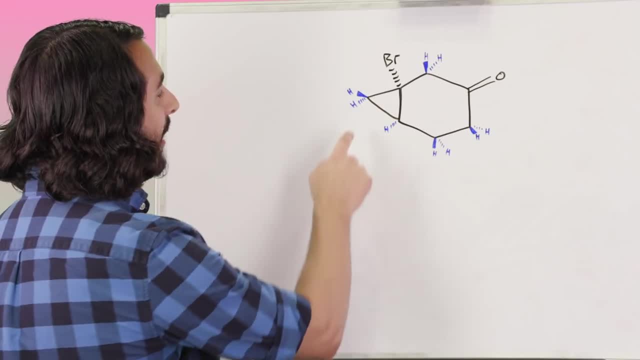 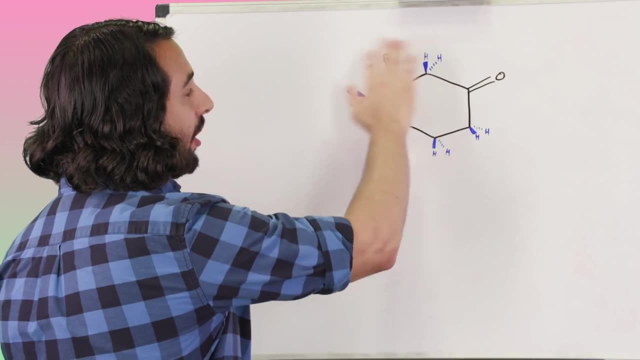 replace one of them with some other element. so let's say we put a fluorine here versus a fluorine there, we would be generating a chiral center because of the other structure on this molecule. there are other groups there, other functional groups, and so if we put